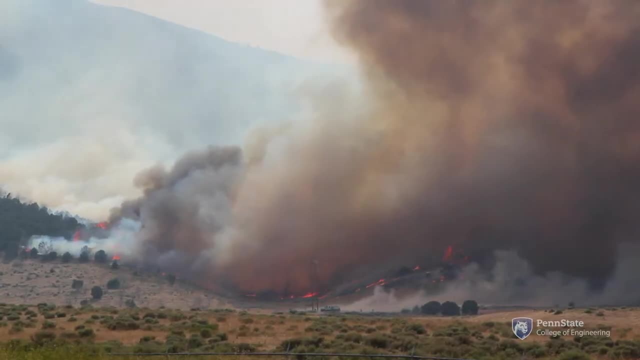 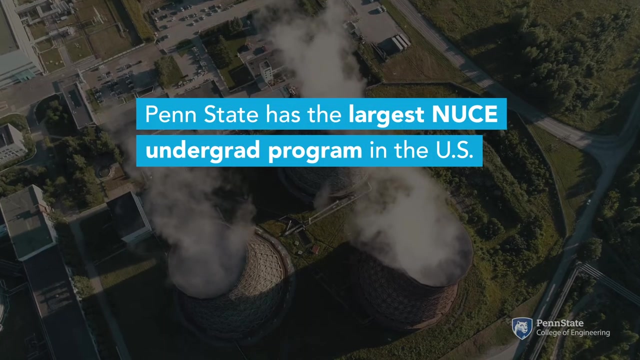 energy for sustainability and to address climate changes as a carbon-free energy source. Many go on to graduate school, after which they work in academia, industry or at research laboratories. Penn State's Ken and Mary Alice Lindquist Department of Nuclear Engineering houses the Brazil nuclear reactor the longest. 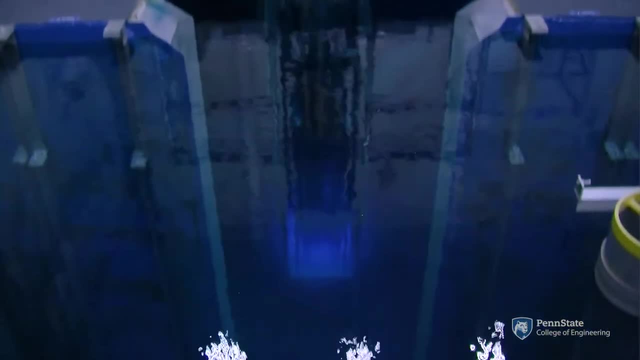 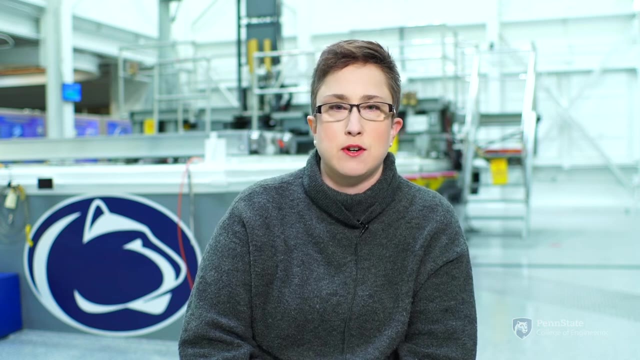 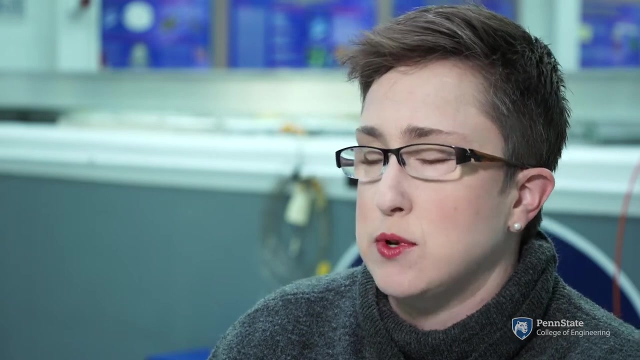 operating licensed research reactor in the country. Faculty and students alike use this reactor to conduct research that propels the field forward. Nuclear currently provides a significant portion of power that is clean, carbon-free and with a relatively low waste footprint, And I think in the future, as we look to get off of fossil 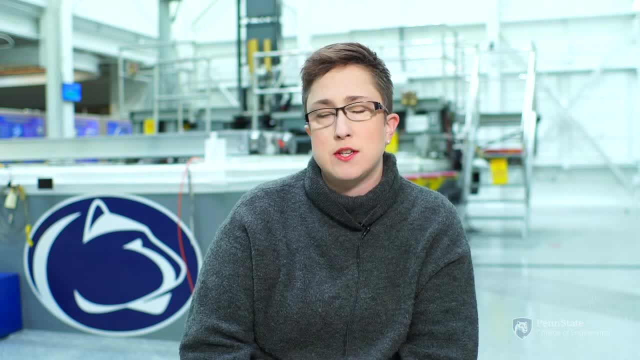 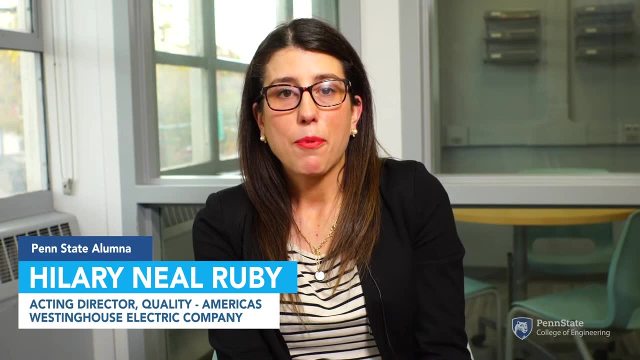 fuels and bridge the gap to new technologies. I think nuclear is going to have to play a huge role in that. What I love about being a nuclear engineer is just the opportunity to interact with people, to solve problems and to really work in a global context. The nuclear engineering field is growing pretty rapidly. It used to only be a power engineering field, but now we have a lot of ties in the medicine materials labs and other places, even propulsion, as the space industry starts to come back. 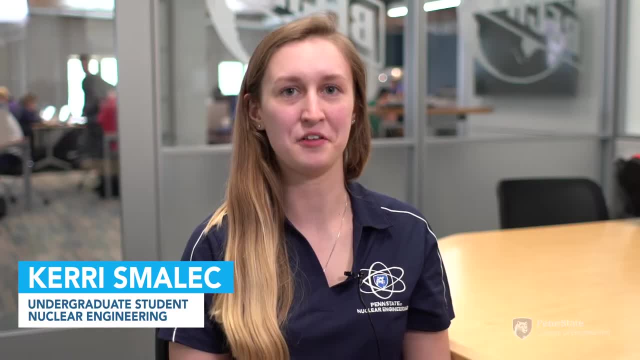 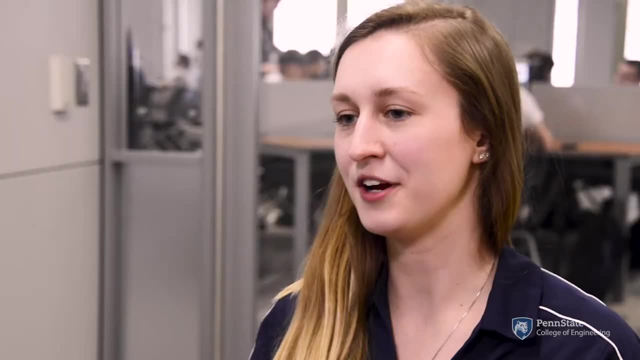 I kind of knew I always wanted to be in STEM. I saw the Incredible Hulk got hooked, saw Iron Man, and Iron Man became my favorite superhero And I did a little bit of research and found out that his arc reactor that powers his suit was. 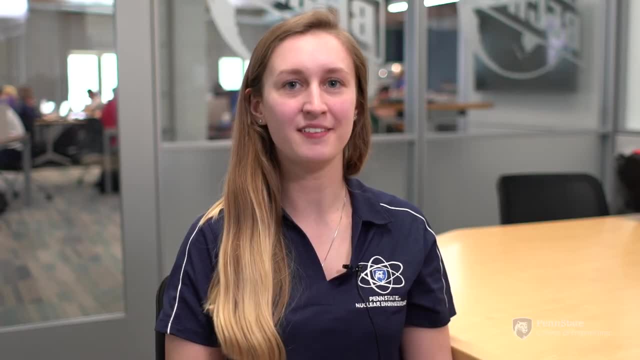 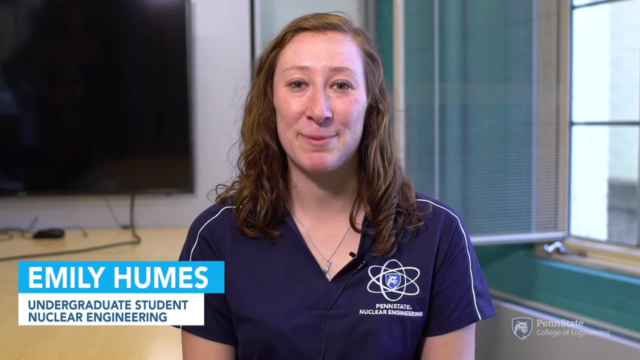 basically a nuclear reactor. So I was like: I want to build the Iron Man suit, I'm going to become a nuclear engineer, and here I am. One of the aspects I love most about being a nuclear engineer here at Penn State is that our class sizes are typically smaller than most larger. 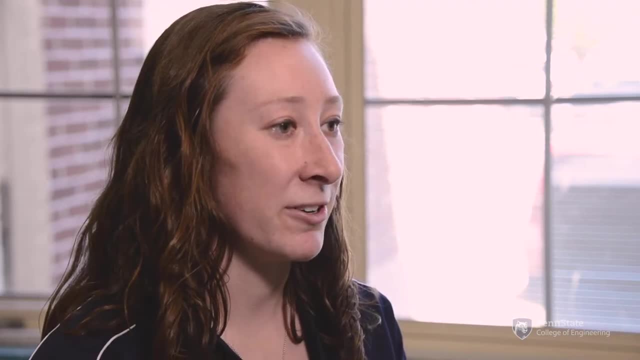 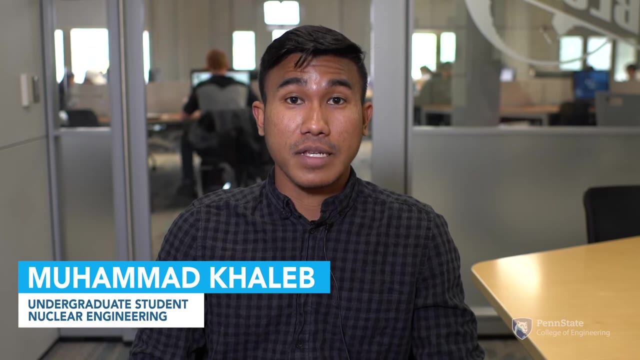 engineer classes. So you really get to know everyone in your major on a one-to-one basis and you make all these meaningful connections with the people around you. There are a lot of research for undergrads in nuclear engineering. So if you talk to your professor, 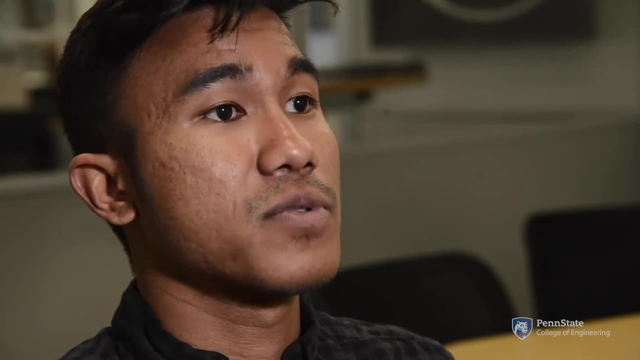 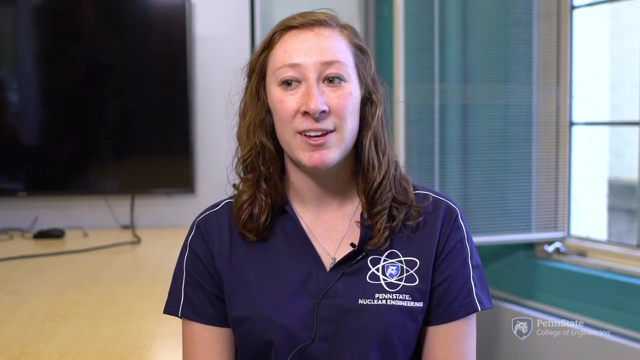 and you hand in your resume, they would more like you to accept you doing your research As a nuclear engineering student. you can actually have the opportunity to work part-time at the reactor on campus. You can become an auxiliary operator so you can help prepare samples, load them into the different test tubes, help move the